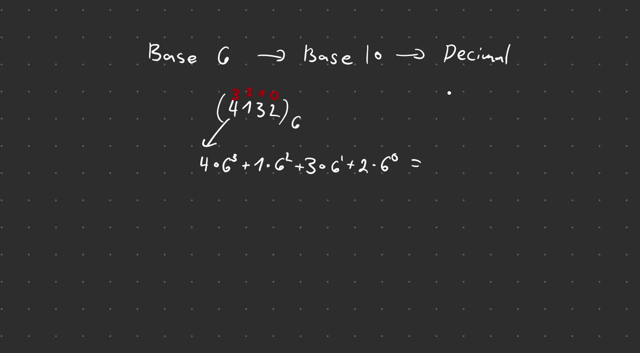 So let me just go ahead and do the calculation real quick. All right, so our number is going to be 920.. All right, perfect. Now one more question: What do I do if I have a number that has a decimal point after? 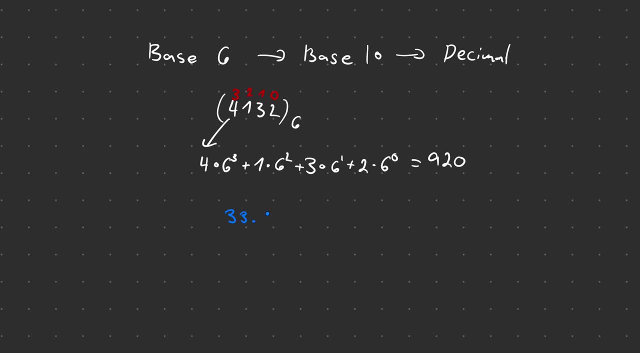 So, for example, let's say we have 33.503, for example, Okay, so this is in base 6 now And it has, And it has, a decimal point. So what we're going to do is quite the same, you know. method. 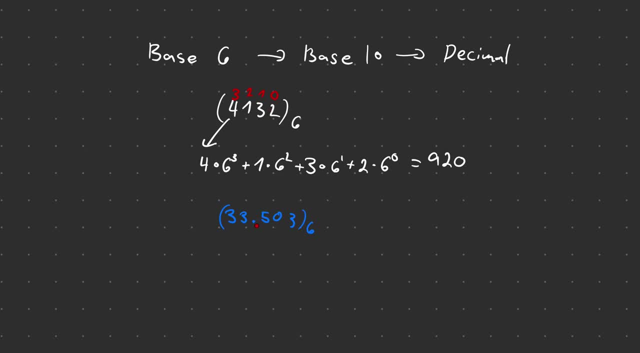 So I'm just going to, over here, write down our indexes. So now what we do is we look at the decimal point and we're going to start our zeros from the first number to the left after the decimal point. So that's 0, and this is 1,, just like we did here. 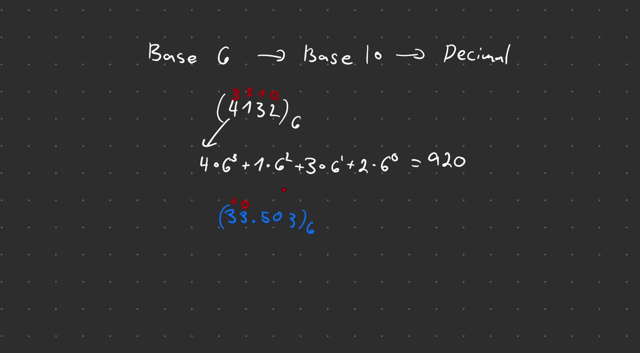 And if there were more numbers here I'd do you know: 2,, 3,, 4, etc. Then, after the decimal point to the right, what we're going to do is just put a minus 1, minus 1, minus 2, minus 3.. 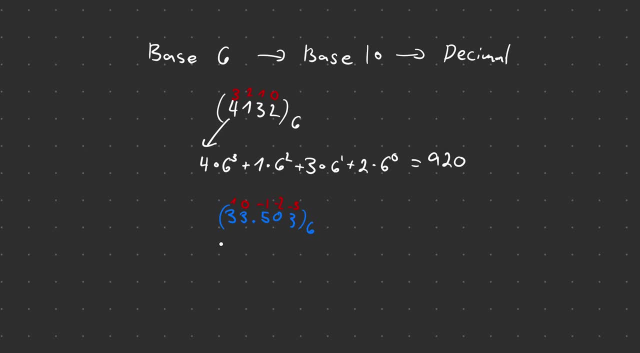 Now what we do. what we're going to do next is the exact same thing for the numbers without the decimal, And I'll show you how to do that right now. So we do 3 times 6 to the 1th power, plus we take this 3, now 3 times 6 to the 0th power. 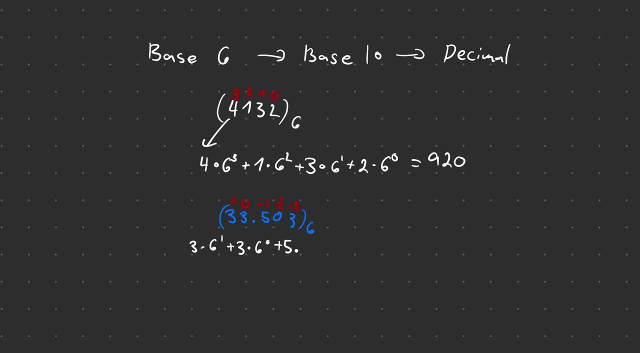 Then we do plus, and then we take this 5,, 5 times 6 to the negative 1 power, And then we plus 0, and whatever, 0 times No, I'm just going to write it down: 0 times 6 to the minus 2 power. 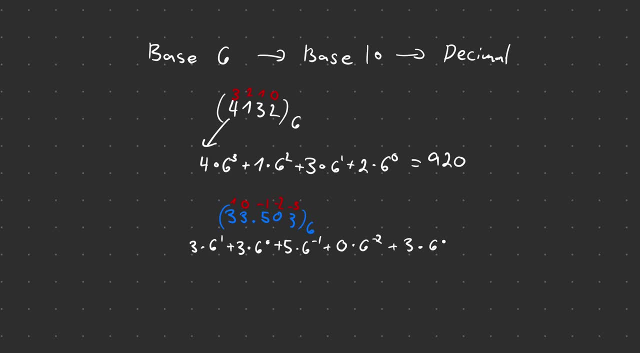 And then we're going to take this 3 here and put 3 times 6 to the negative 3 power. Now, if we do this calculation, we will get our decimal value of this number. Thank you very much for watching this video. If you enjoyed it, please feel free to subscribe and have a great day.